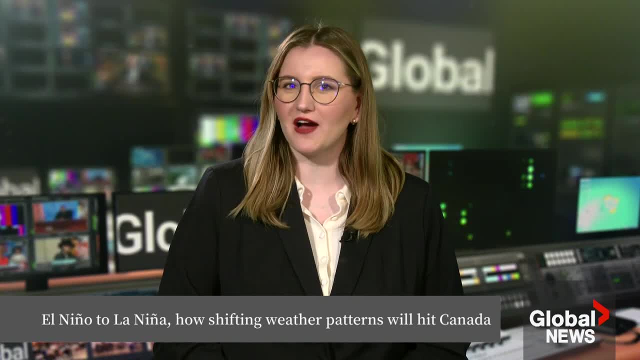 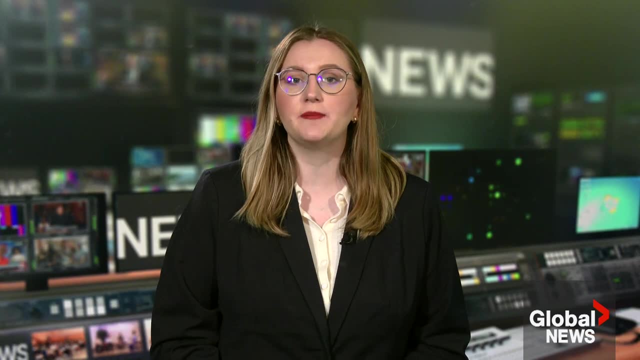 If you put away your scarves and mittens this winter, make sure you have them handy next year. Meteorologists are predicting that a chilly La Nina event is on its way and could begin as soon as July. La Nina happens when sea temperatures are cooler than normal. 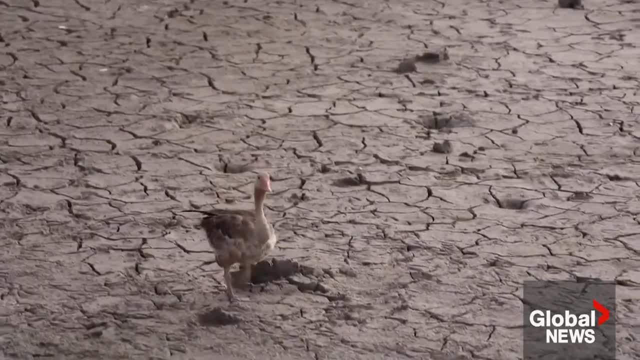 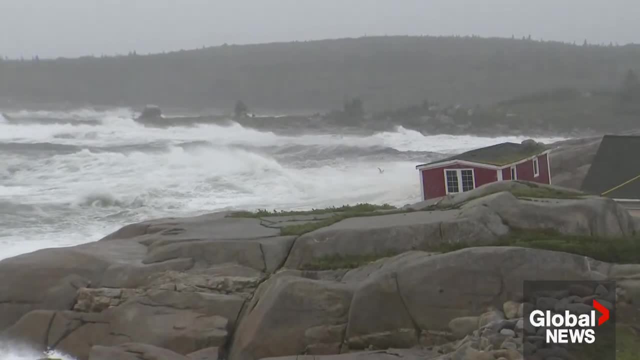 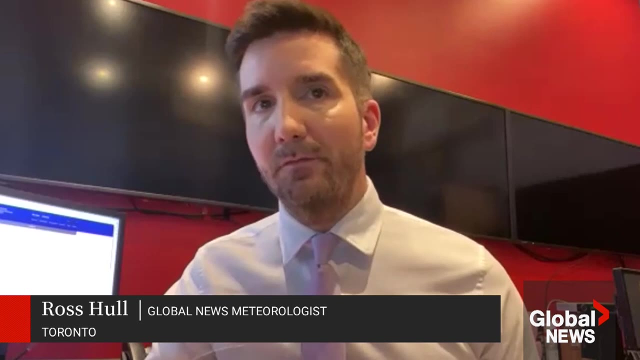 El Nino is the opposite, causing the warm temperatures being felt in Canada since June. Oftentimes these events affect more than just the weather, which is why global news meteorologist Ross Hull says they have to be under close observation. What happens when you see changes in the ocean temperatures above normal or below normal? that can have widespread impacts, what we call teleconnections to other meteorological factors like jet streams and storm track and precipitation, even hurricane development. The events typically last between 9 to 12 months, but Hull says that time frame has been getting longer. 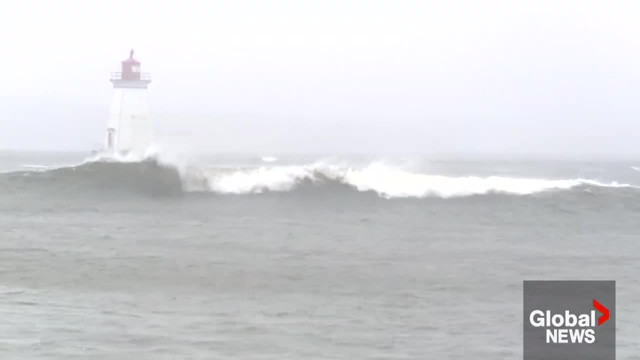 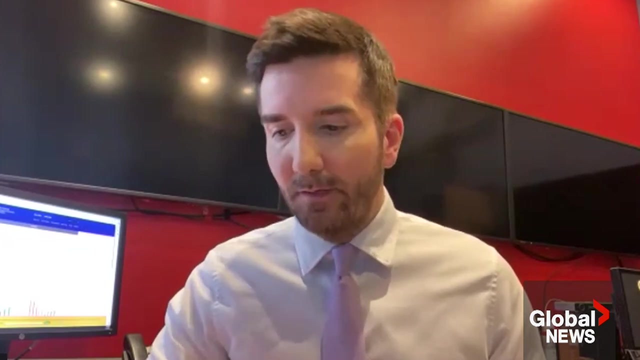 The previous La Nina spanned nearly three years and there were consequences. When you look at that period between 2020 and 2022, there was certainly a heightened amount of Atlantic hurricane season activity, According to the Columbia Climate School's research. 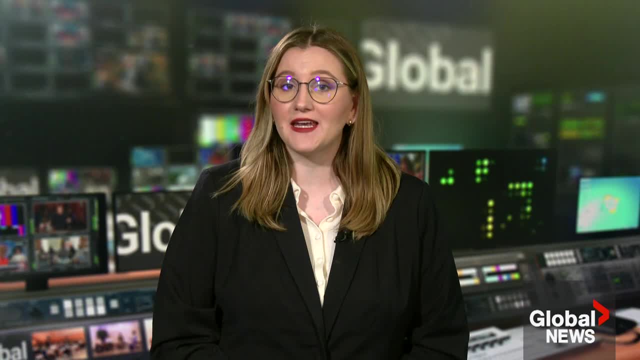 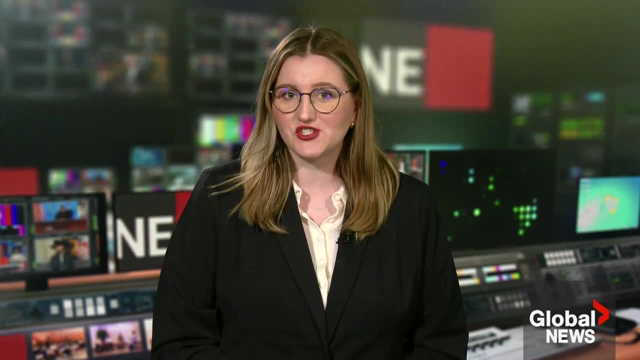 there is a 58% chance of a La Nina event beginning this year. Hull says Canadians in the West Coast, Ontario and Quebec can expect greater levels of precipitation. In terms of hurricanes, he says it's too early to tell How strong La Nina's signal will be. Naomi Bargiel Global News. 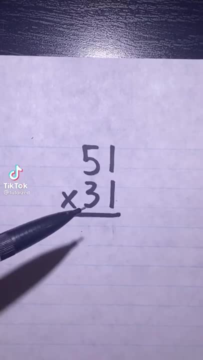 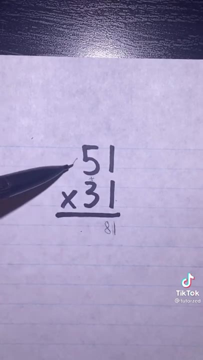 This math trick makes multiplication so much easier. Alright, so if we're multiplying two numbers ending in one, all we have to do is put one at the end, add the first two digits together and put that in front of the one, and then multiply them and put them in front of that. 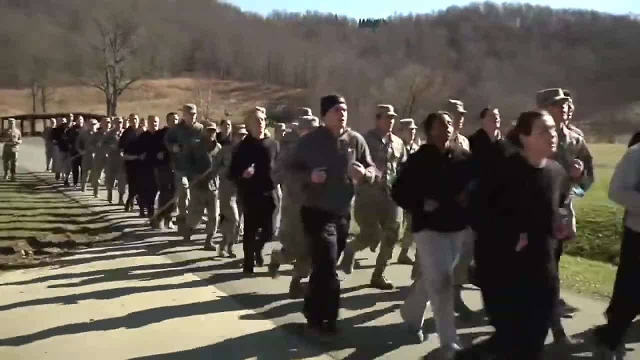 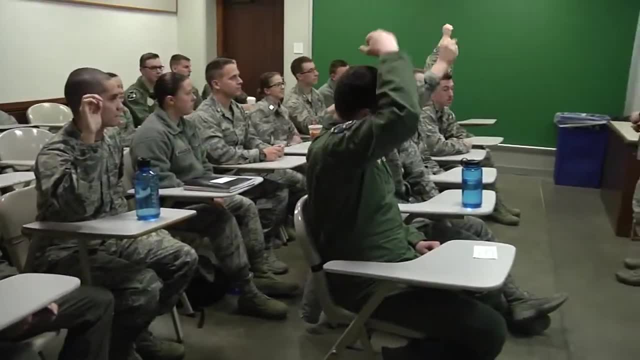 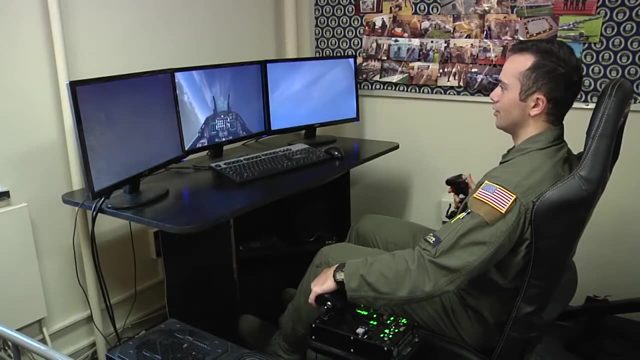 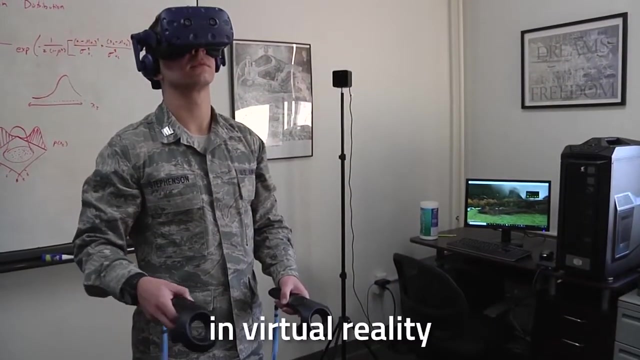 In Air Force ROTC, we aren't just strong, We aren't just tough, We aren't just smart, We are innovative, developing new solutions, leveraging cutting-edge technology and making positive contributions to society. At Detachment 730,, we are developing real-world tools and virtual reality. We are using VR to 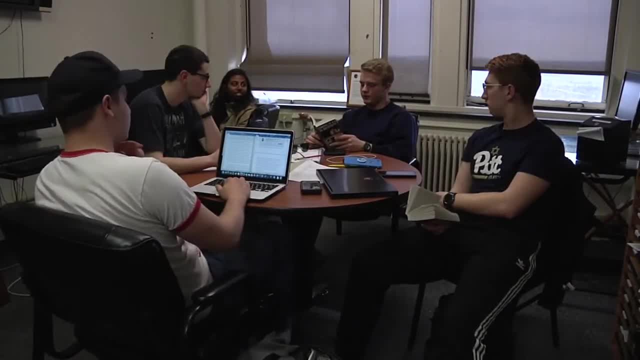 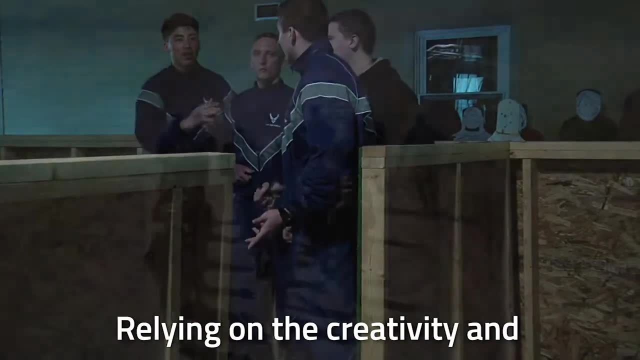 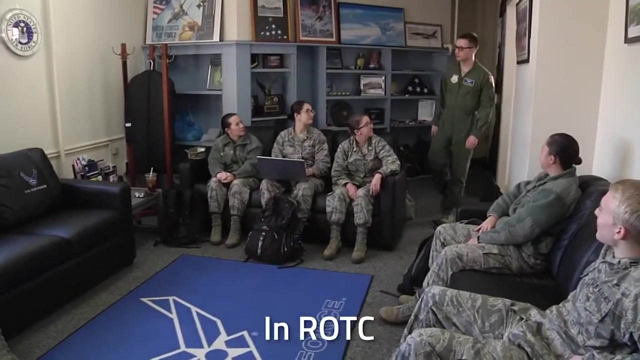 assist STEM cadets and support our academic tutoring program. In the future, our cadets will create new solutions relying on creativity and problem-solving skills they develop through ROTC. In ROTC, the opportunities are endless. Are you ready to put your creativity and